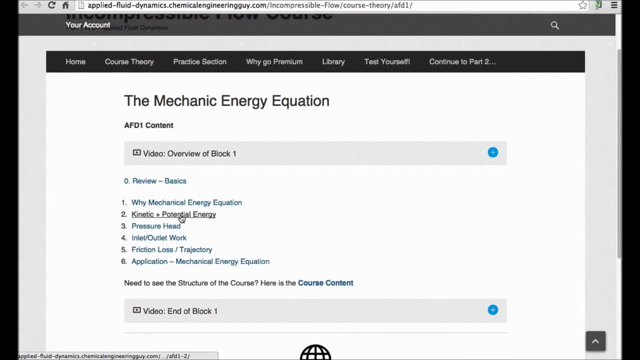 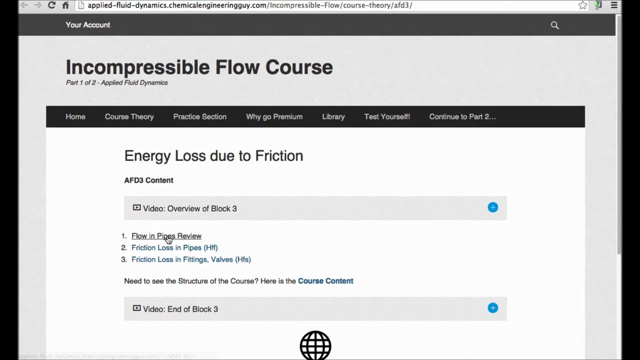 Mechanical energy equation is all that is: momentum, transport, Kinetic potential, energy pressure, head inlet, outlet works, frictions and so on. Then we start once again with the theory: what is a pipe, materials, and so on. We start calculating pipe losses and fitting losses, essentially friction losses and pressure drop. 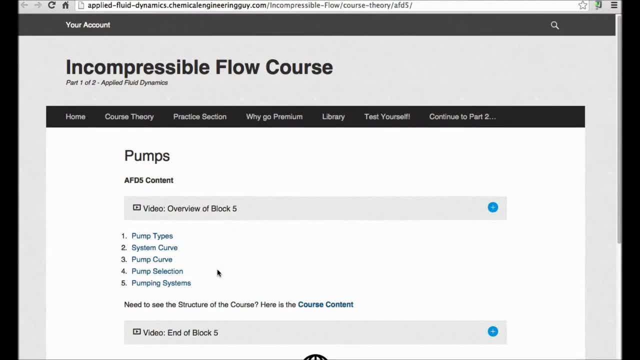 Then the venturi tube, orifice blades and many other devices. Then, finally, we start analyzing types of pump: what is the system curve, pump curve, how to select the best pump for the system And, eventually, which type of pumping system there are. 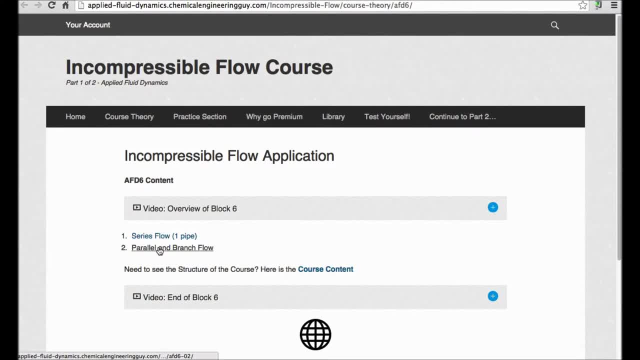 Then we analyze series flow, which is a very important concept, And then we check out parallel flow and a little bit on branch flow. Finally, agitation and mixing. a little bit on theory, design of equipment and software, modeling and static mixtures. a little introduction. 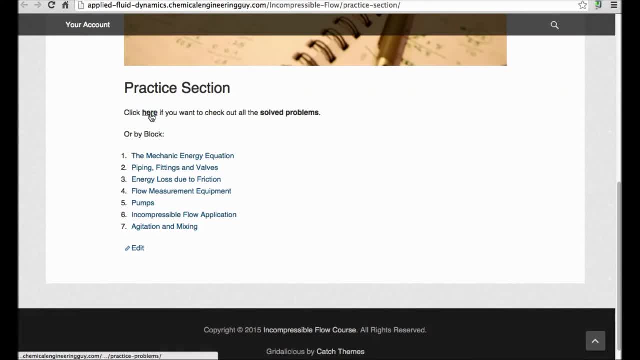 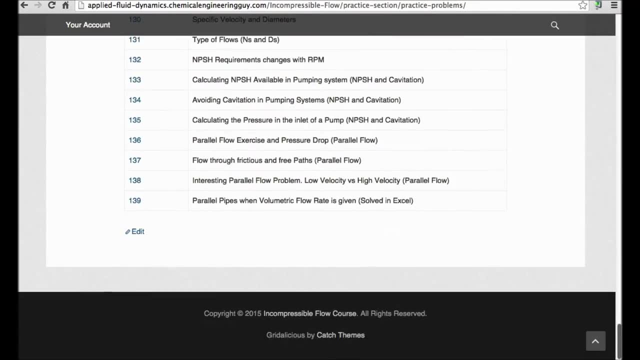 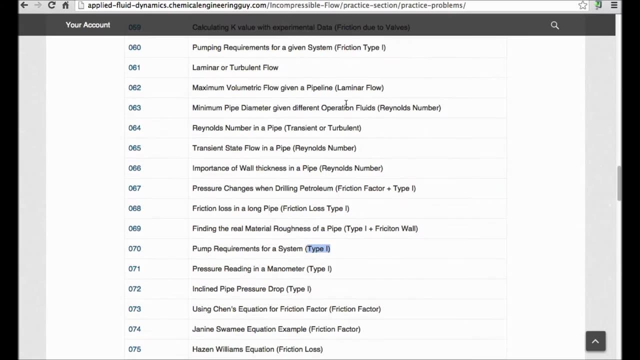 And all this is supported with practice. And then we have problems and solve problems. video problems so you can check out. there are 140 problems all related here: choosing pumps, power of a pump, friction loss, Taiwan problems, which is serious problems and transient and turbulent. we got Reynolds number and we got also Bernoulli's and to reach all this law, 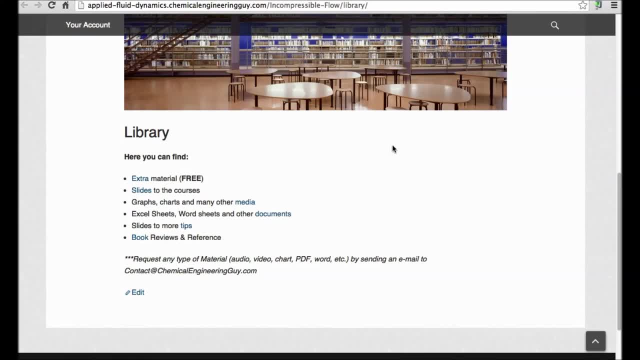 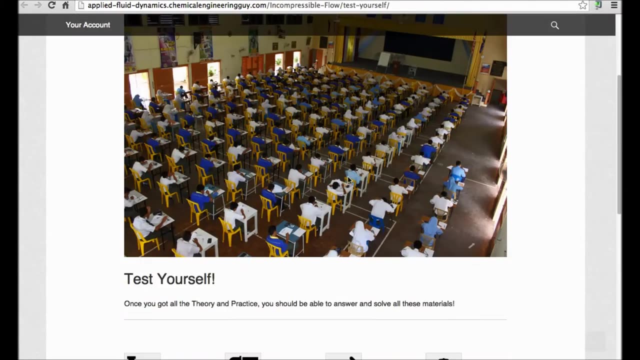 To show you this library, which is essentially just for where to get slides. I got you graph charts and many other things. There are all here: Platt-Lindsen paper, media, Excel, water sheets- I prepare for these documents, some tips and the book reviews of the related. 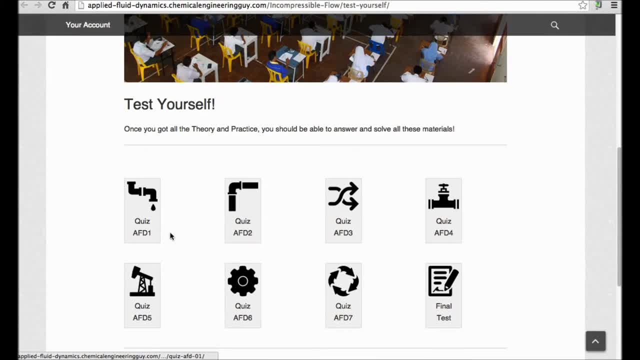 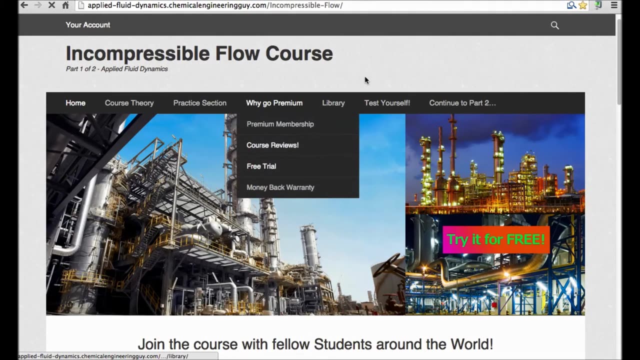 The test yourself section, which is essentially just questions, theoretical questions on what you were studying before. This is about all the seven blocks I told you and we got a final test. You can always go and check out the free trial. Doesn't cost you any money, it's free. 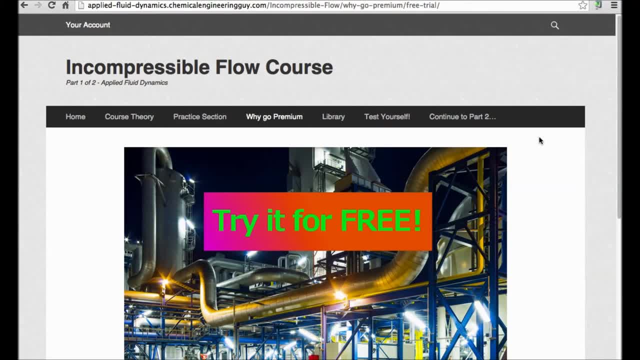 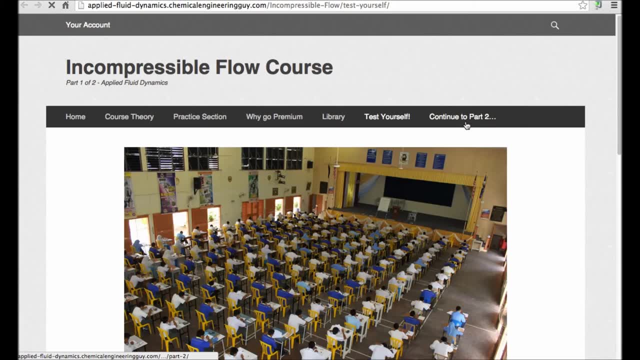 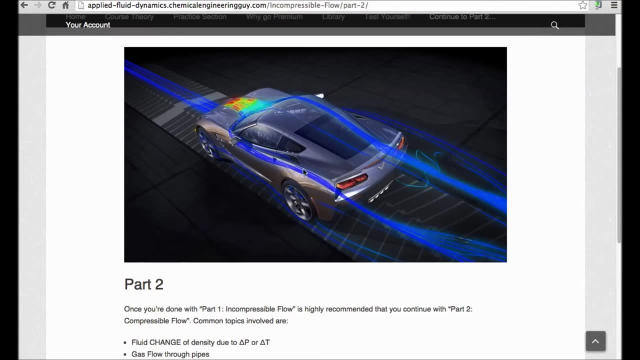 for three days and if you think it's good for you, you can enroll to all the other courses. now, Once you're done, you can continue with part number two, which is compressible flow- essentially what happens when you have a gas rather than a liquid. and if you enroll into part number one, you will get a 50 discount.